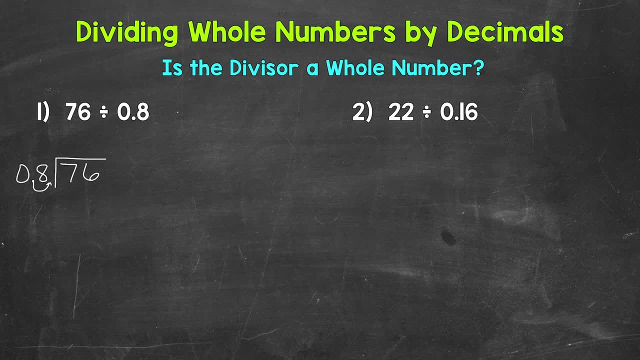 For example, number one, we multiplied 8 tenths by 10. That shifted the digits one place to the left, therefore giving us a whole 8.. But we made that process a little simpler to think through by just thinking of this as moving the decimal to make the divisor whole. 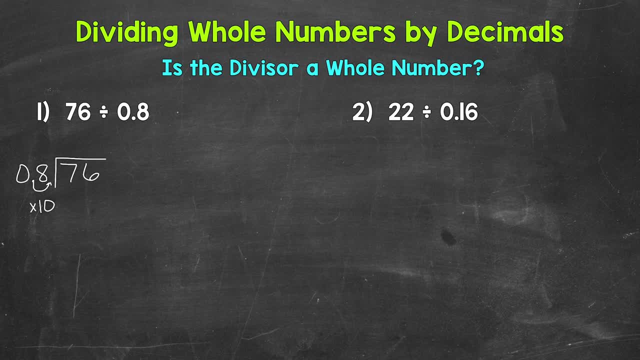 Now what? Whatever we do to the outside, the divisor, we must do to the inside, the dividend. So if we multiply the outside by 10, we need to multiply the inside by 10 as well to keep this problem balanced. So let's move the decimal once to the right on the inside. 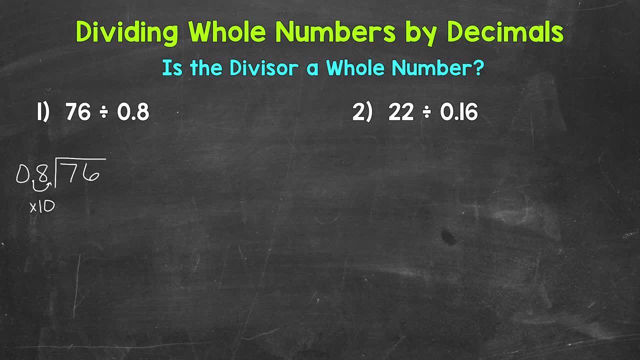 Now 76 is a whole number, so the decimal comes after 76 and any other whole number. Let's move it once to the right, fill this with a 0, and we multiplied our dividend by 10 as well. Now that we have our whole divisor, let's rewrite this equivalent problem to the side. 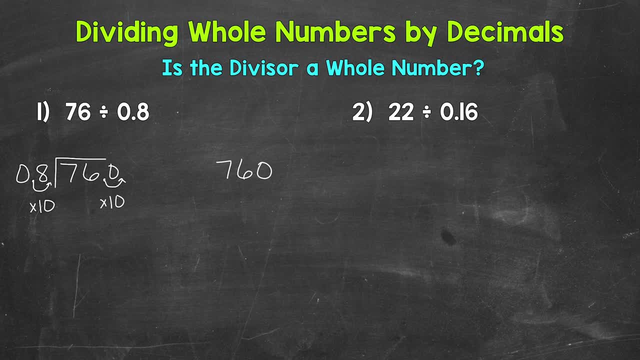 So we have 760 divided by 8.. Now our divisor is whole, so we can go through the division process. So divide, multiply, subtract, bring down, repeat. Let's start with divide. So we have 7 divided by 8.. 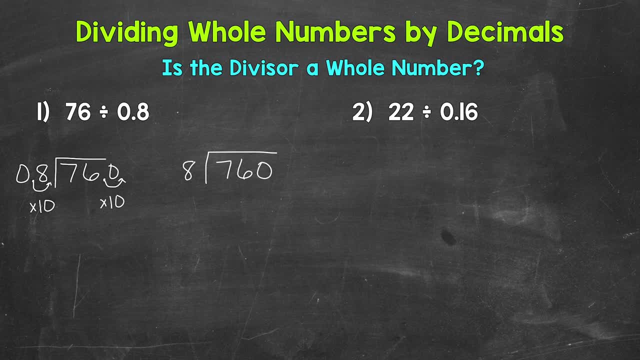 How many whole groups of 8 in 7?? Well, we can't do that, So we need to use the 6 and take a look at 76.. 76 divided by 8.. How many whole groups of 8 in 76?? 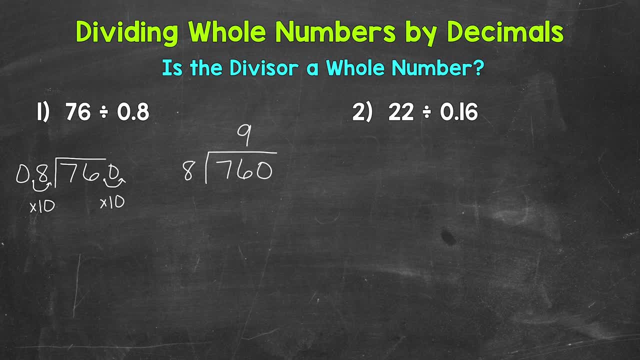 9. That gets us to 72. And that 9 needs to go above the 6,, not above the 7,, because we used 76 there. Now we multiply 9 times 8? 76. 72.. 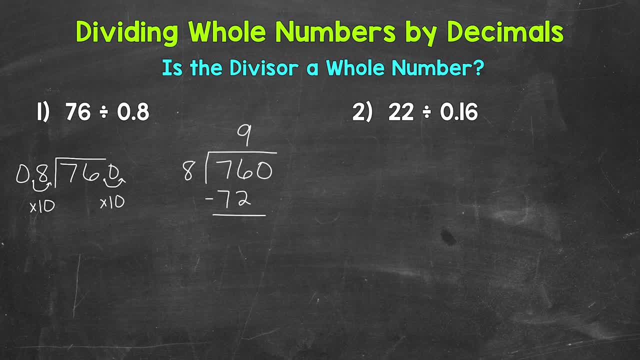 Subtract 76 minus 72 gives us 4.. Then we bring down And then repeat. So we go back to divide. Now we have 40 divided by 8. How many whole groups of 8 in 40?? Well, 5.. 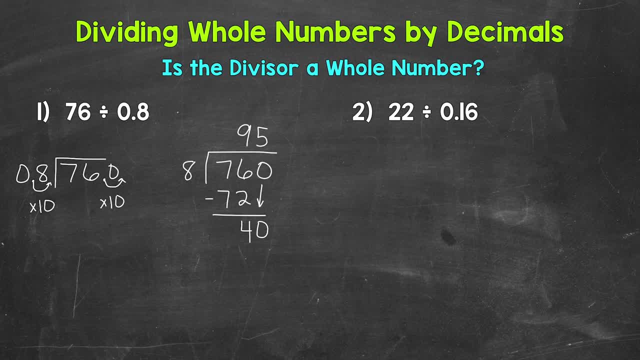 That gets us to 40 exactly. Multiply 5 times 8? 40.. Subtract 40 minus 40? Is 0.. We went all the way over to the furthest place to the right. We have a clean cut 0 at the end here. 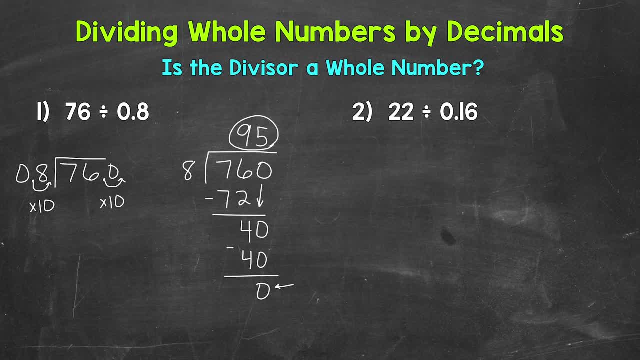 So we are done. Our final answer: 95.. Now for number 1, we have a whole number answer. We went all the way over to the furthest place to the right in our dividend as far as bringing digits down, And we have a clean cut 0 at the end. 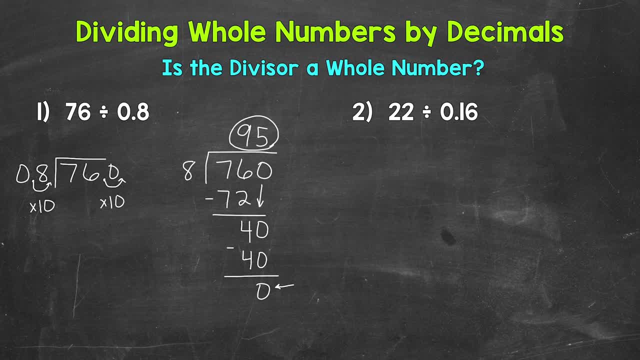 So we do not have a decimal part of our answer. Again, we have a whole number answer In number 2,. we will see what happens when we do have a decimal part of our answer. Let's move on to number 2, where we have 22 divided by 16 hundredths. 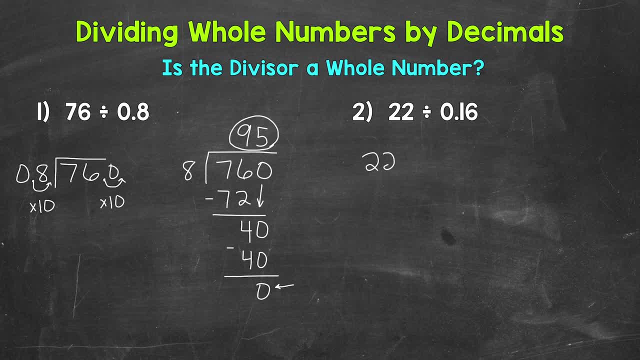 Let's set this problem up. So we have 22.. That's our dividend, the number we are dividing, And then 16 hundredths is our divisor, the number we are dividing by. Is the divisor a whole number? Is the divisor a whole number? 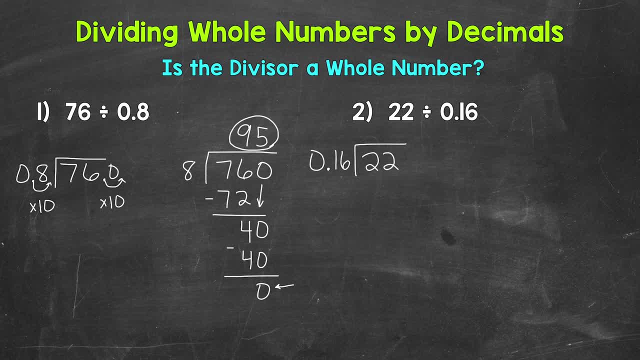 16 hundredths is not a whole number, So let's make it a whole number by moving this decimal twice to the right, And that's going to be a whole 16 now. Now, technically, we shifted the digits of 16 hundredths two places to the left. 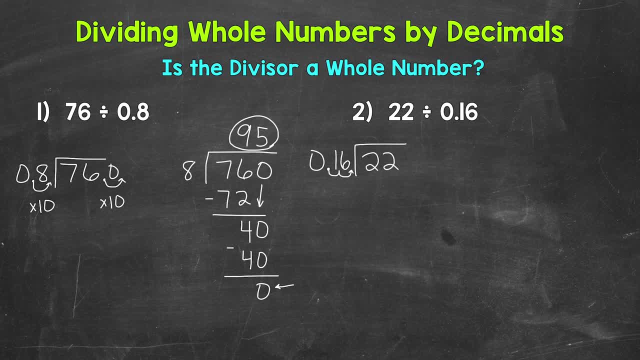 to make that a whole 16.. The power of 10 that we multiplied by was 100. Now, since we multiplied the divisor by 100, we need to multiply the dividend by 100. Let's move that decimal twice, So the decimal comes after 22.. 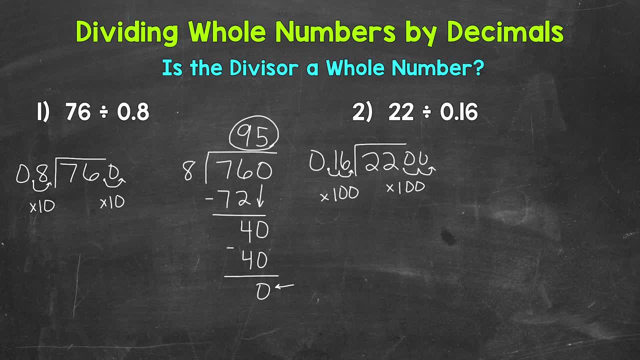 Once twice fill those gaps with zeros And we have our equivalent problem that we can rewrite and solve. So we have 2,200 for our dividend divided by 16 hundredths. So we have 2,200 for our dividend divided by 16 hundredths. 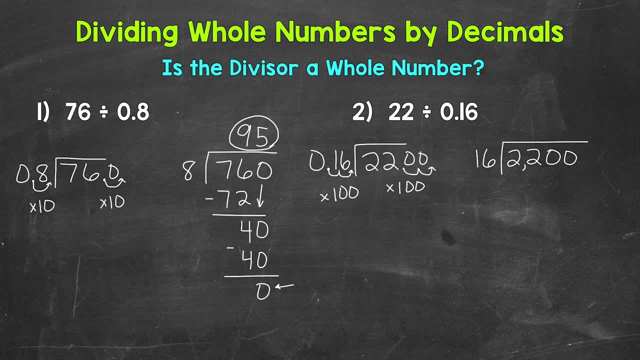 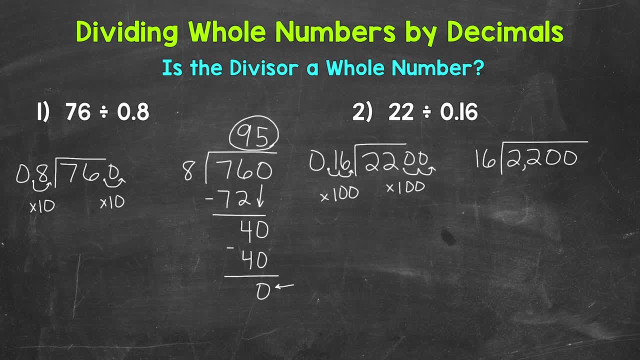 So now our divisor is whole and we can go through our process. Start with divide, So we have 2 divided by 16. How many whole groups of 16 in 2?? Well, we can't do that, So we need to use 22.. 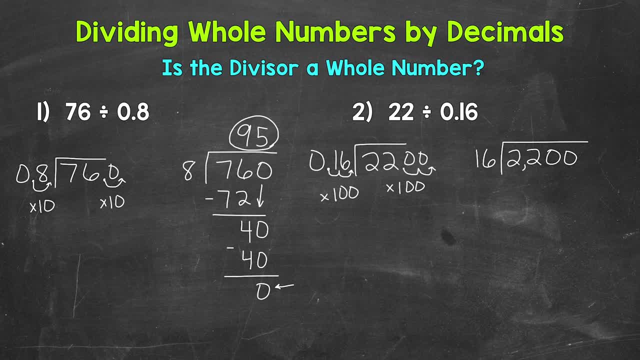 22 divided by 16.. How many whole groups of 16 in 22? One That one needs to go above the 22,. not that first two, since we used both of those digits and took a look at 22.. and took a look at 22.. 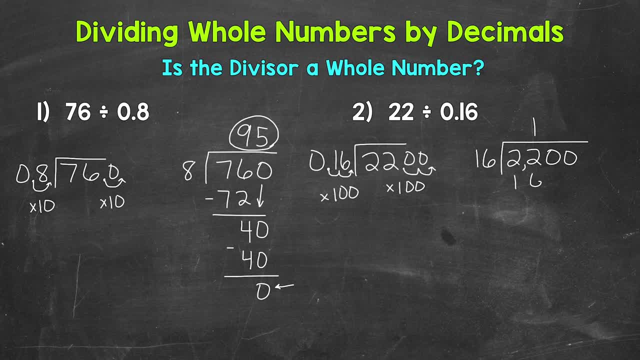 Now we multiply One times 16 is 16.. Subtract: 22 minus 16.. Let's borrow: It's a 1 there, And we have 12 minus 6, which is 6.. And then 1 minus 1 is 0.. 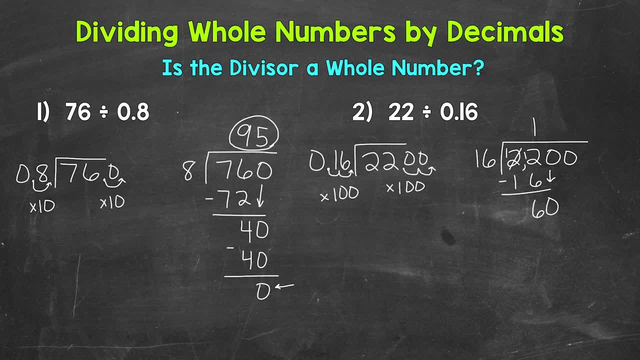 Now we can bring down this 0 and we have 60. So we need to repeat and we go back to divide: 60 divided by 16.. How many whole groups of 16 in 60?? Well, 16 times 3 is 48.. 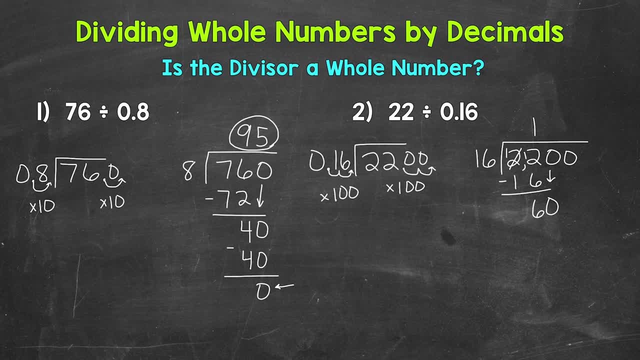 16 times 4 is 64.. 4 is too many, It's going to be 3.. Multiply 3 times 16.. 48. Now we subtract So 60 minus 48.. 0 minus 8.. 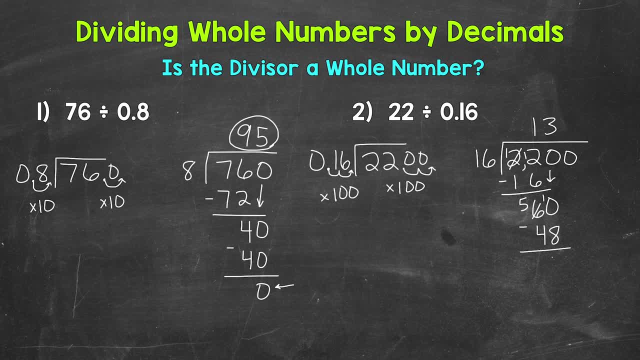 Well, we need to borrow here: 10 minus 8 is 2.. And then 5 minus 4 is 1.. So 60 minus 48.. 48 equals 12.. Let's bring down that next 0.. Now we repeat: 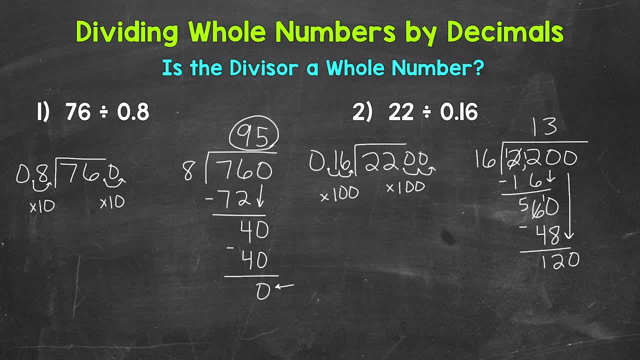 So we go back to divide. We have 120 divided by 16.. How many whole groups of 16 in 120?? Now, you may not know how many whole groups of 16 are in 120 using mental math, So we can estimate and check in order to find out. 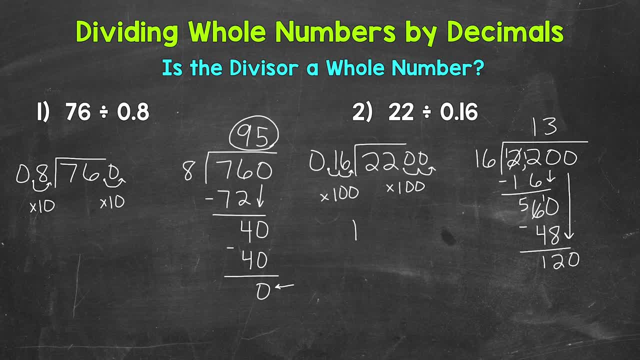 So I'm going to come to the side and use 16.. 16 times 10 as our reference point. So our starting point 16 times 10 is 160.. That's kind of close to 120.. So we can adjust based on that. 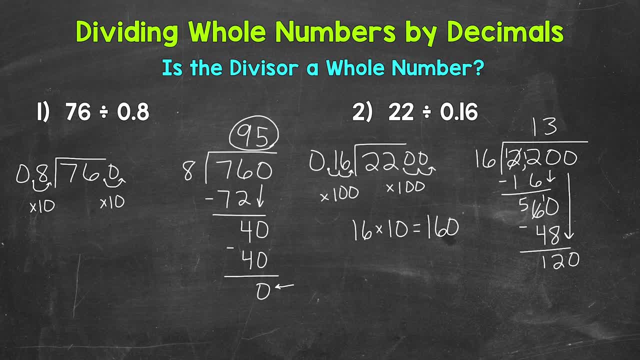 Let's try 16 times 8 and see how close to 120 we get 16 times 8.. So 8 times 6.. 48.. 8 times 1 is 8.. Plus 4 is 12. 128.. 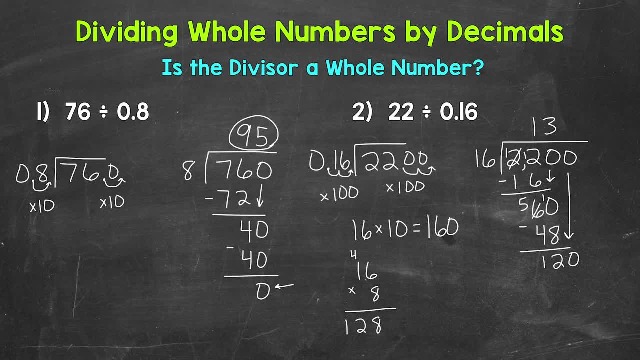 So 8 groups of 16.. That's too many. Let's try 7.. 16 times 7.. 7 times 6. 42. 7 times 1.. 7 plus 4 is 11. 112.. 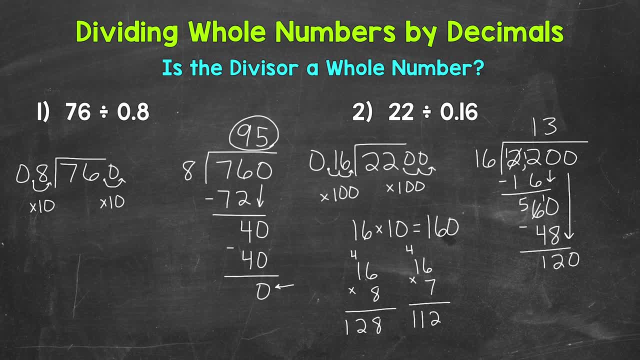 So it's going to be 7 groups of 16.. Let's put our 7 up here. Multiply 7 times 16.. 112.. Subtract 120 minus 112.. Let's start with 0 minus 2.. 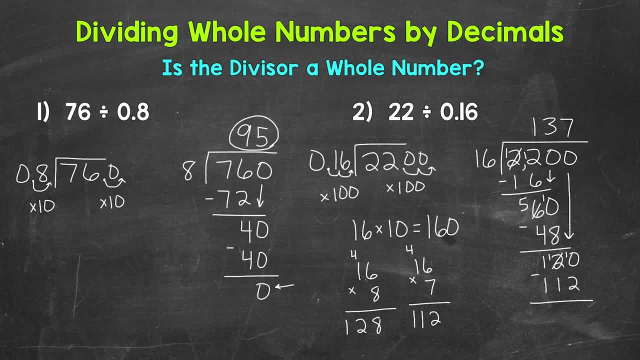 We need to borrow. So that's 10 minus 2, which is 8. And then we have: 1 minus 1 is 0. And then another 1 minus 1, which is 0. So we end up with 8.. 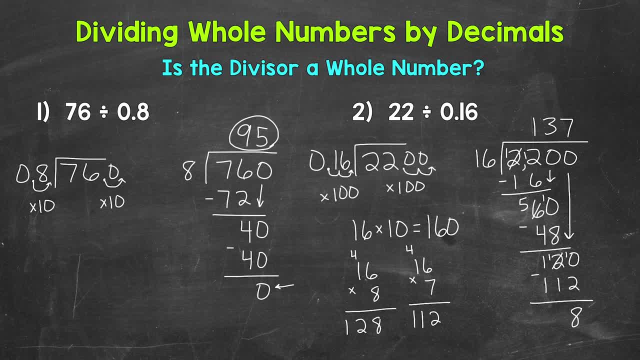 Now we went all the way over to the furthest place to the right. We're going to write within our dividend, So we do not have anything else to bring down. But we do not have a clean cut 0. at the end We have an 8.. 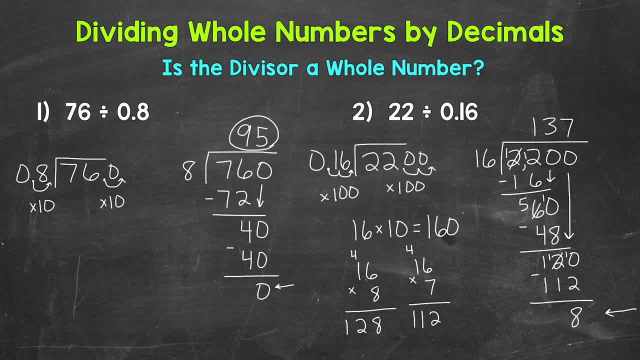 We do not want to write 137 remainder 8.. We are working with decimals, So we want everything within our problem to be in decimal form, including our answer. So we need to continue this problem until we do get a clean cut: 0.. 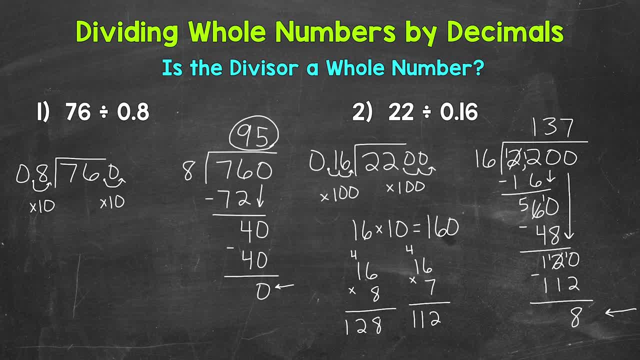 So what we can do, We can include the decimal In our dividend And then bring it straight up into our answer. Now we need something to bring down in order to continue this problem. So what we can do, We can use placeholder zeros to bring down. 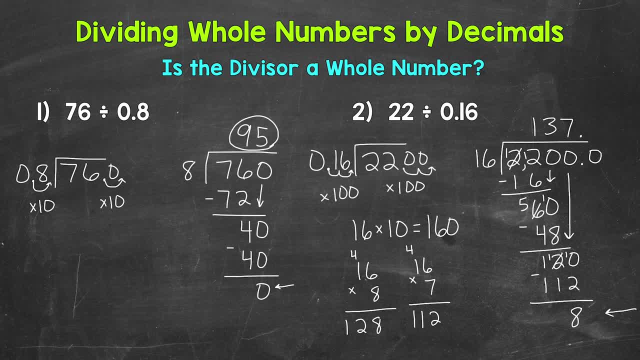 Remember, zeros to the right of a decimal or decimal digits do not change the value of that number, So we are able to use this strategy in order to continue the problem. Let's bring this Zero down And continue the problem. Now we have 80..